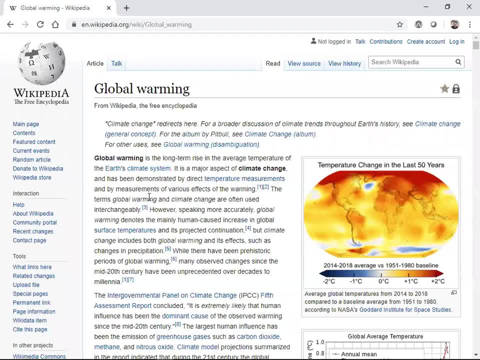 And this you can basically apply to any Wikipedia page. So this is the Wikipedia page that I'm actually using, And here I can see that there is something written about global warming. So I'm going to pick up or scrap this whole content and later on I can create a word to web. Already I've uploaded a tutorial on word to web, and you can do many more things. You can also convert all these particular sentences into words, But now in this particular video we'll try to focus on how to do a web scrapping for this particular page and get that data and how you can convert this into sentences. 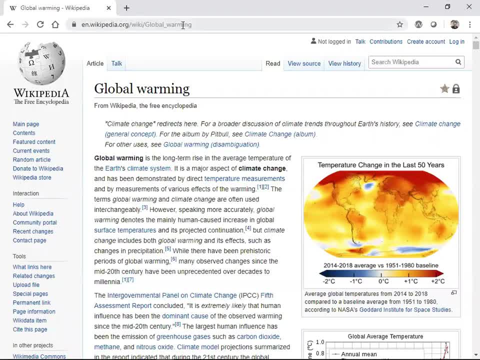 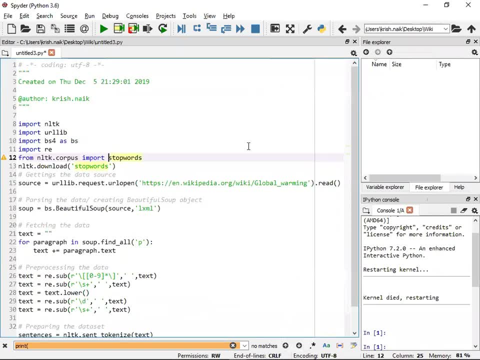 So that is the plan. So this is basically my URL that I'm going to use. I'm going to web scrap from this particular URL as we go ahead with the help of beautiful soup. So let us go ahead. So, first of all, let me just zoom in this code. Now, the first thing that I'm going to use is an NTK library, because if I'm reading some text data, if I have to do some text pre-processing, I'll basically be requiring this kind of library. Apart from that, I'm also going to use beautiful soup. Okay, so for that I'll be importing BS4.. So if you don't have this particular library, you can just say conda install. 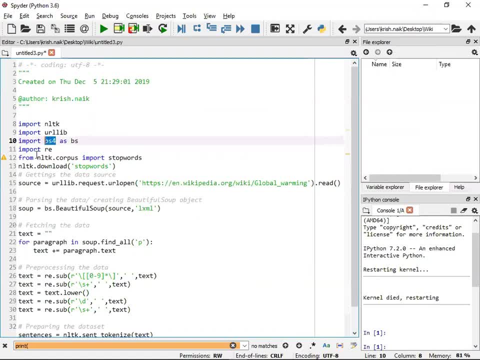 BS4, it'll get already imported into your from your Anaconda prompt. try to run this particular command. Apart from that, I'm also going to import RE, which is called as regular expression. I'm also going to use stop words because I suppose I want to clean this particular text by removing some unnecessary words like to from the his, which is not required, you know, to just do the sentiment analysis. I can basically remove this. And again, guys, here I'm not going to perform any sentiment analysis, but I'm trying to basically use a beautiful soup and I'll try to do that. 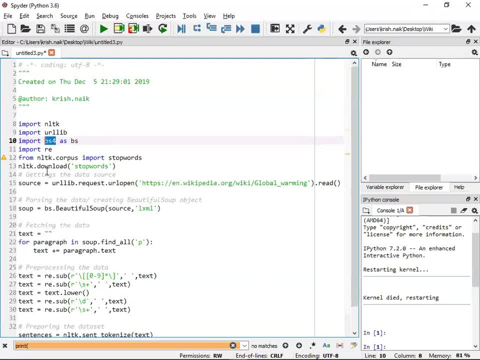 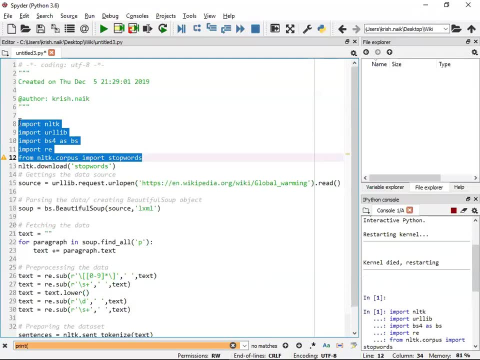 I'm going to try to show you how we can scrap this page. That is my Wikipedia page over here. So first of all, I'll just import all these particular libraries. Okay, that is required, And this is. this will be a small tutorial, because many of you have actually requested how we can basically web scrap a page, But if you want the complete tutorial, please do let me know in the comment box. I'll try to create this whole tutorial for web scrapping, along with deployment, you know, by using Heroku platform and all. 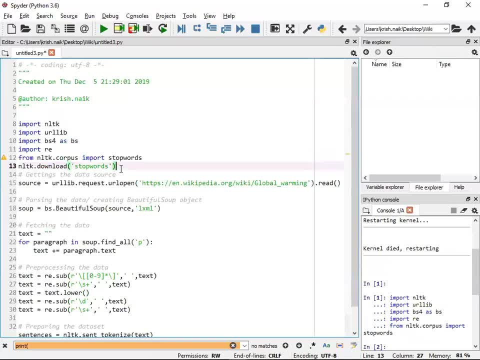 So here it is. So I don't have to execute this download stop words, because I've already executed and I have all the all the stop words present. But even though, if I execute, you can see that it is saying that I already have this particular data, So it is showing us true right Now. in order to import the text from this URL, all I have to basically use is something called as URL lib, which is my library over here: dot request dot URL open. Okay, now, when I'm using this particular dot request dot URL open, I'm going to use the URL. 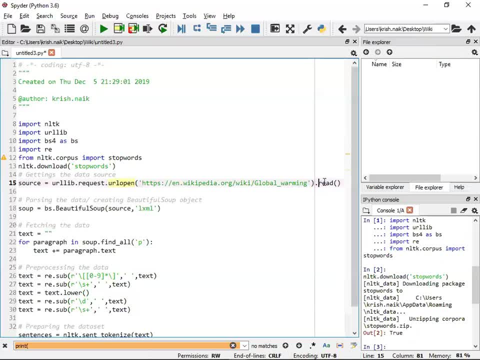 that I want to read and I have to use the dot inbuilt function called as dot read. right, So URL lib, dot request, dot URL open. I have to just provide the URL page And when I say dot read, I'm basically going to get the content of the entire HTML And later on, what I'm going to do is that I'm going to initialize this DS4, that is, BS dot, beautiful soup. And always remember, guys, beautiful soup requires two parameters. One is the source and how we basically want to parse the text data. So here it is. 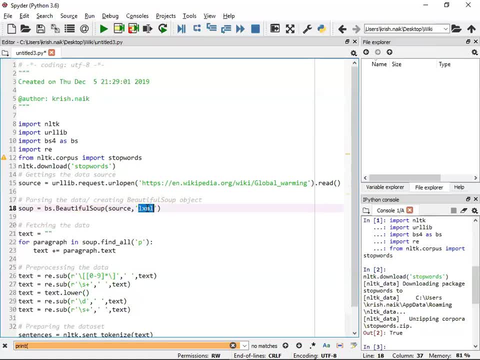 Here I'm going to basically use that use as LXML, so that you know, we'll be able to apply various for loops to read the data inside that particular text And this is how one technique we can basically do the parsing. that is LXML. 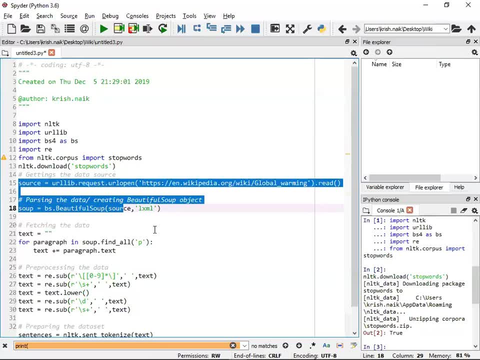 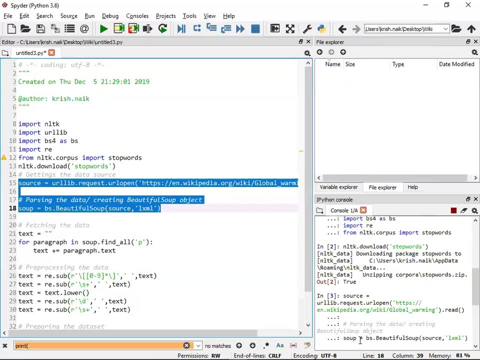 Now you can see that as soon as I execute this, I'm going to execute this two line. So here it is. It has got executed perfectly. Now you can see that it is taking a little bit time, but that's fine, Yeah. 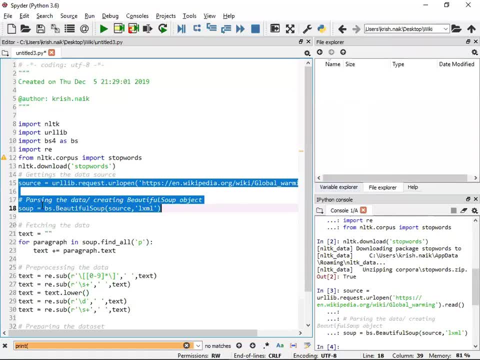 Now I can see this. Still, variable explorer is not created because SOAP is just an object, a parsing object in SHA. Now, what I'll do is that? remember, guys. let me just go back to the webpage and show it to you. Suppose this is my webpage. 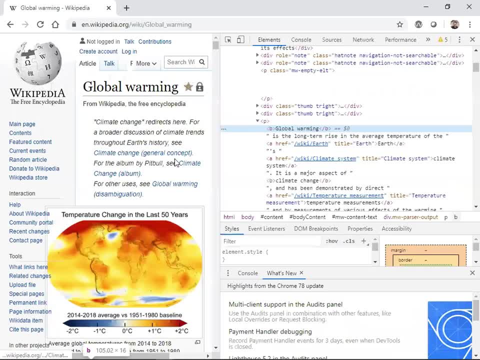 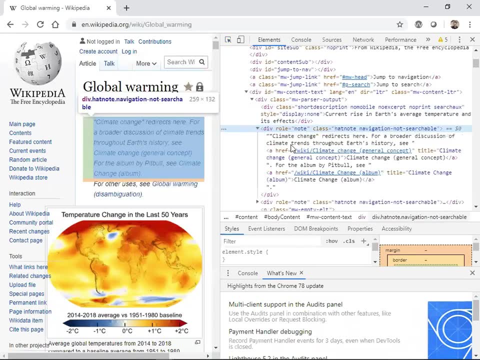 Here you can see that if I just inspect this global warming right, you can see that it is present inside p tag. Okay, Everything is present inside p tag. So if I go inside div, there will be a p tag to actually pick up all the information. 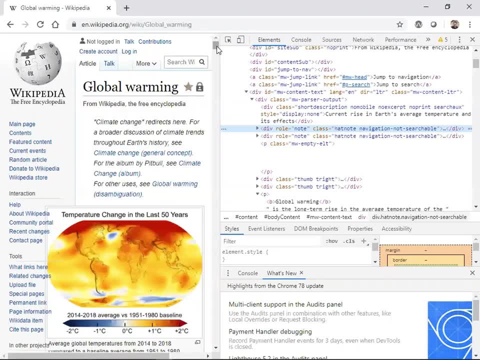 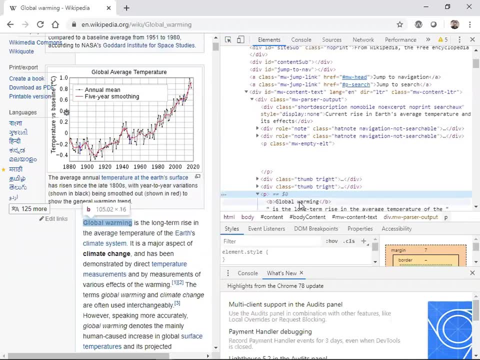 Okay, I'm not going to take this, So instead, What I'll do is that just let me scroll down. Okay, So once I scroll down, suppose I want to pick up this particular data. right, You can see that it is inside the p tag. 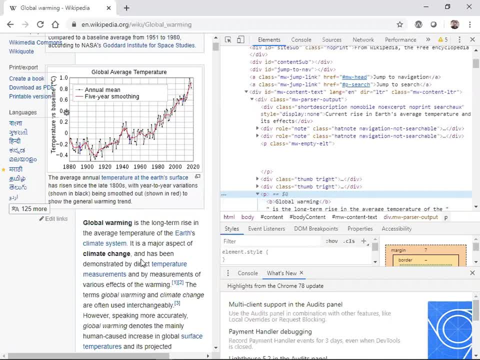 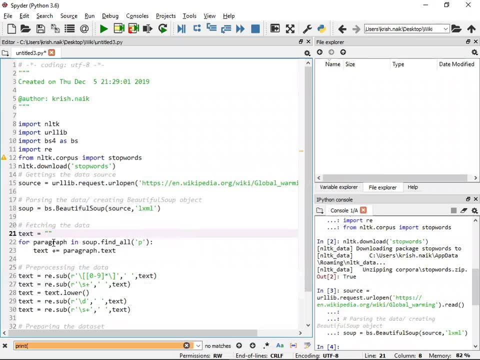 So what I'm going to do is then I'm going to pick up this whole content inside the p tag And I'm going to basically retrieve it over here. So for that, what I'm going to do is that I'll just write for paragraph in SOAP dot. 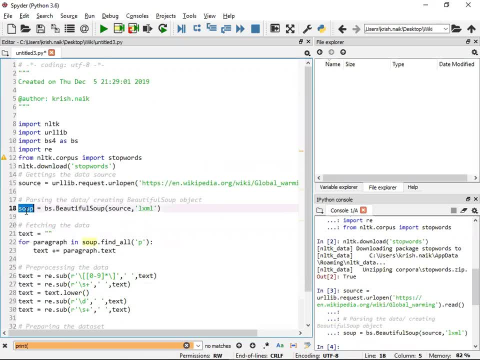 find all. So this SOAP object is basically the parsed HTML data, which will be in the format of LXML, And then What I'm going to do is I'm going to use a p tag which is called as find underscore all. 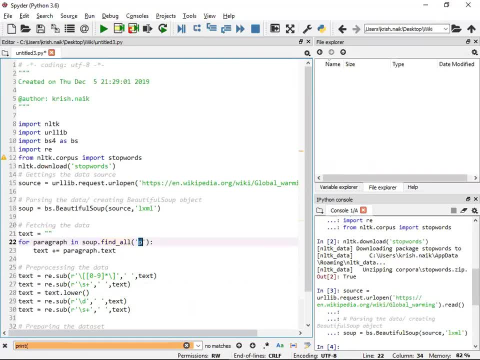 And here I'm using a paratag. Okay, So p tag. wherever there is a p tag, I have to just get the content. for getting the content, I just have to write paragraph dot text to text property, which will have all the texts. 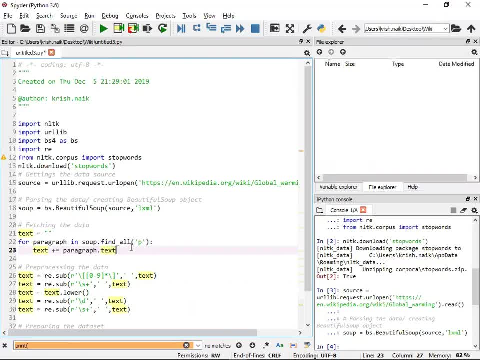 that is present inside this paragraph tag. So what I'm going to do, I'm just going to append it, each and everything. So here you can see that once I execute it. now, if I go and see my text tag, let me just 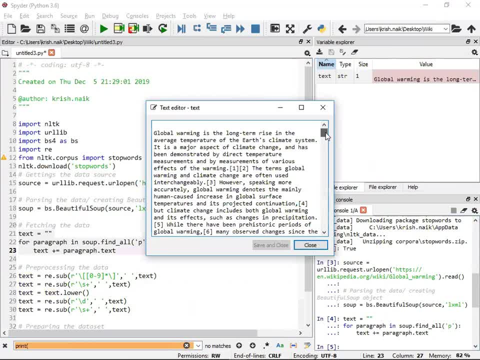 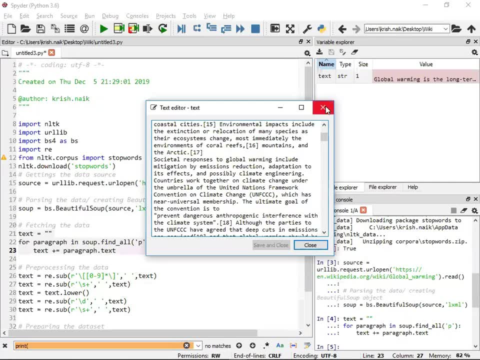 show you. So here it is my text tag. Here I'm getting all this particular information and this is the whole content that I'm actually getting over here. Pretty much simple, guys. I've just used the find all inbuilt method and I have the property over here. 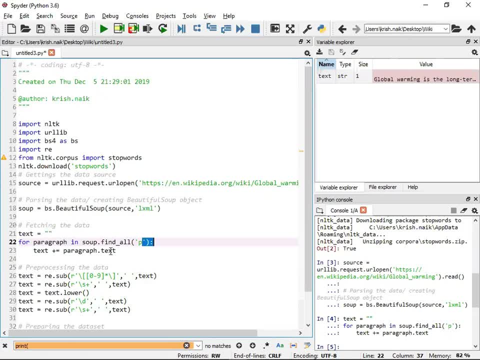 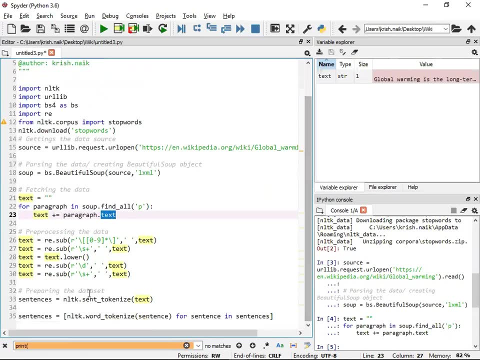 I have the tag which is called as my paragraph tag, And then I'm basically using the text inside that which will have the text inside the paragraph tag. Then after that, you can apply various regular expression Like you want. you want to remove some- there's all characters like one, two, three, you don't. 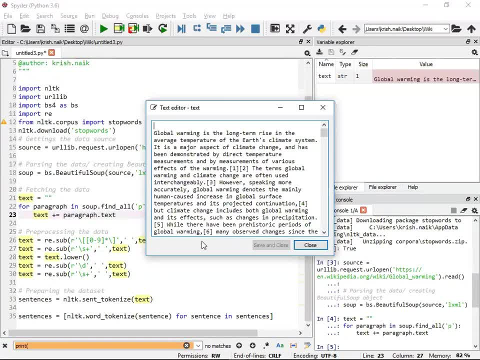 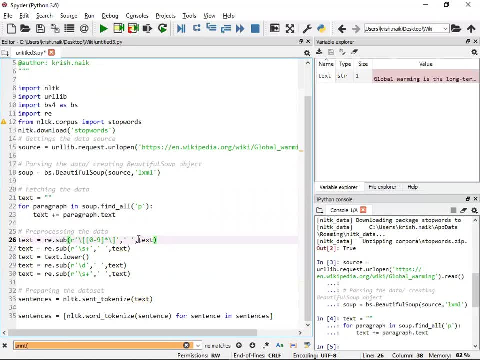 form a full stop. You can apply any type of regular expression. You want to remove that additional spaces. So for that, what I'm doing, first of all, I'm removing all the numbers. I don't want all the numbers in that text, one basically using this particular command. 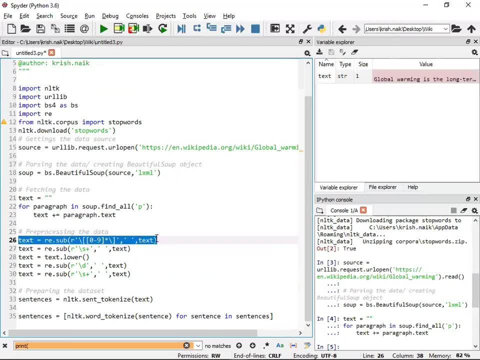 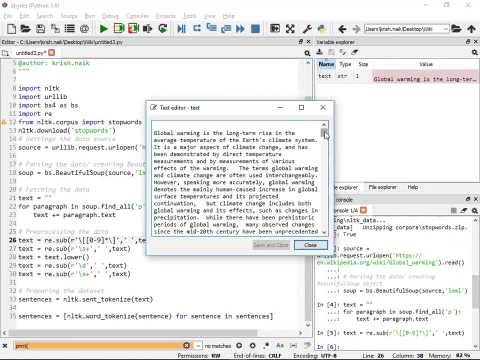 So let me just execute this again and we'll try to see what are the things. And again, for this we are using this regular expression, re. okay, Now, if I go and see my text over here, I see that all that one, two, three characters. 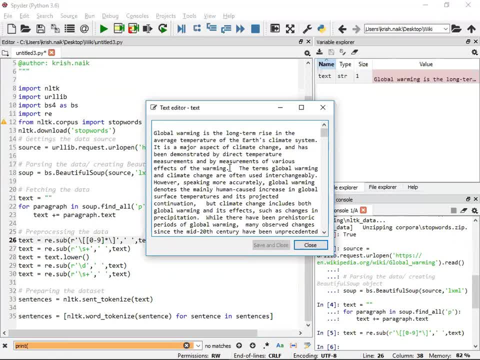 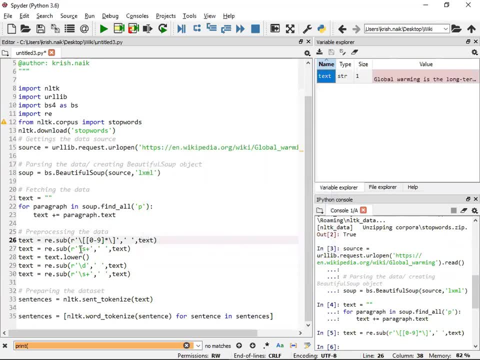 have been removed Right, So it is getting removed. It is getting replaced by a blank space, So this blank space is also not good, So we'll try to remove that blank space. So you can see that additional spaces is being removed over here by using this. 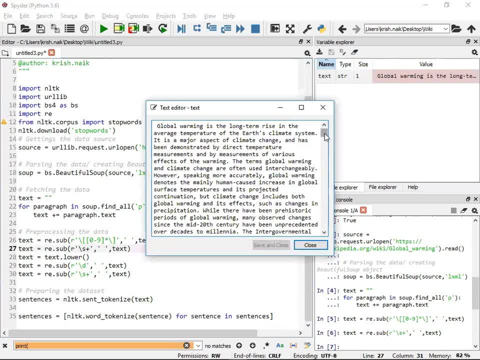 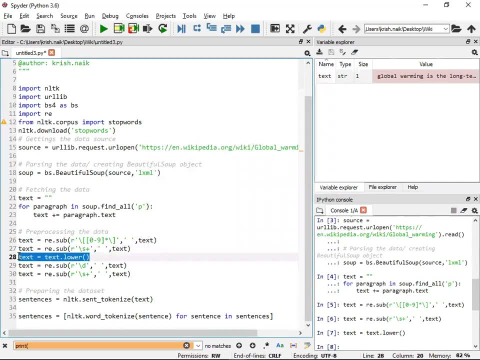 And now I have. you can see that I don't have any blank spaces. right, It is all getting removed very clearly. Here it is Then the next step. what I'm doing? I'm doing the lowering of the text, because there may 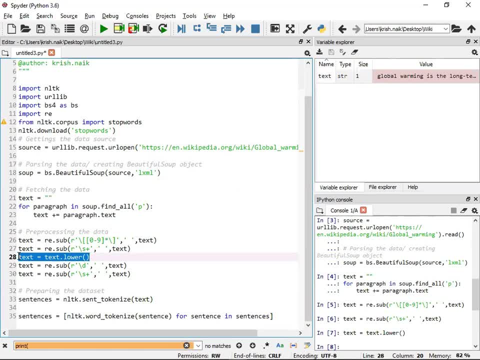 be multiple texts or like it may be, global kind of word. It may be there. It may be capital G, small g, like all this kind of stuff will be there. So let let us make it slower, so it will always be good. 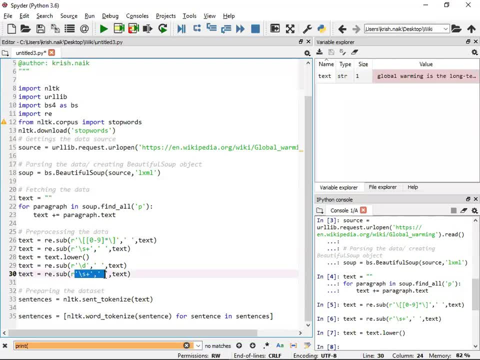 Right, And apart from that. Okay, So this was the code for additional spaces, And again here, I have repeated it again and again, So no need to execute this, And we will execute this also. Finally, what I'm doing is that I'm using NLTK, I'm converting this whole text into 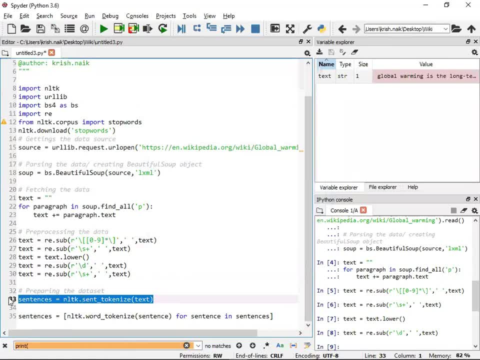 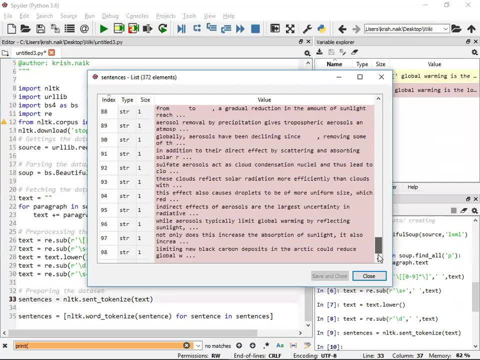 sentences. So, in order to convert this into sentences, I will be showing you now you can see that- the list of 372 sentences and how sentences are basically done with the help of full stop and comma, And that is automatically done by here. 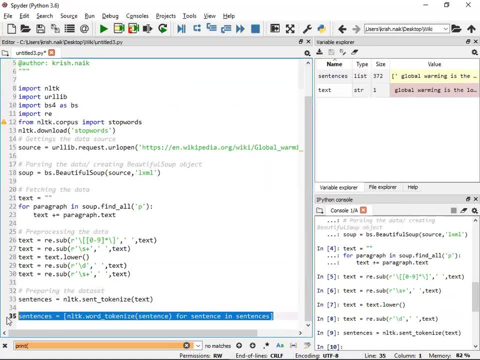 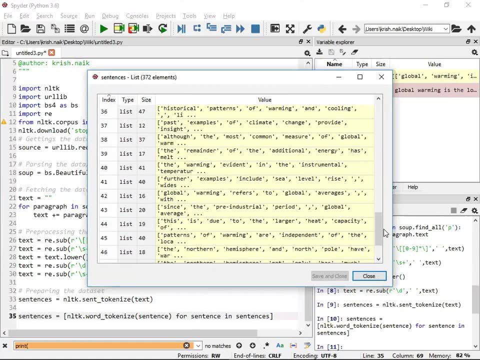 And after this, you can also apply and convert the sentences into words. Now you can see that I'm having all the words by using this particular code, And I have already taken this in my NLP playlist. guys, The main factor is that I needed to show you how we can web scrap an HTML page. 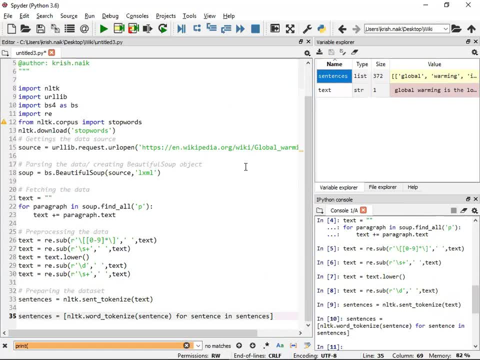 But if you want the complete tutorial on web scrapping with deployment until deployment, please do let me know. I'll create a playlist on that and definitely you'll be able to understand how to do web scrapping, how to do web crawling and many more things. 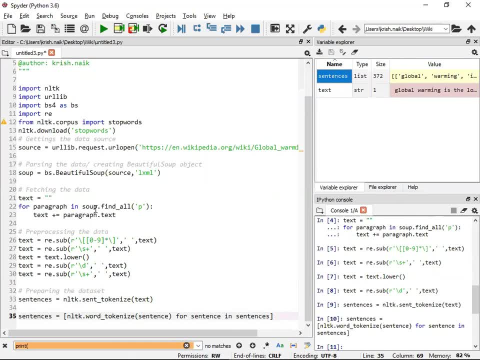 And there I'm going to use this beautiful soup library extensively. So this was all about this particular video. guys, Now if you're looking for career transition towards data science, please make sure that you go and visit Springboard India YouTube channel. The link is basically given in the description. 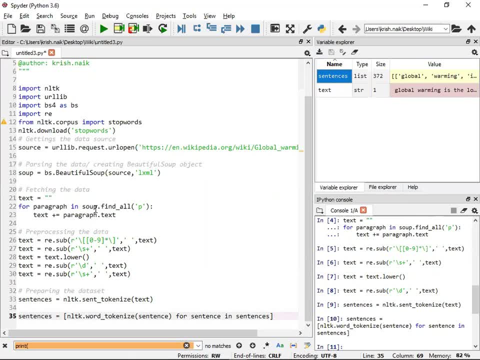 There you'll be able to see the real life talk from data scientists, like how they work, how does the real world project looks like? So, yes, that was all about this particular video. I hope you like this particular video. please do subscribe to the channel if you're not. 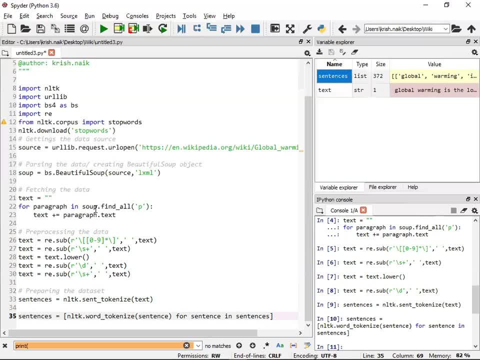 already subscribed. I'll see you all in the next video. Have a great day. Thank you, one down.